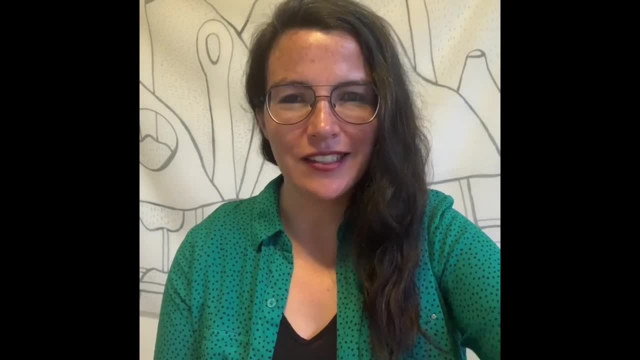 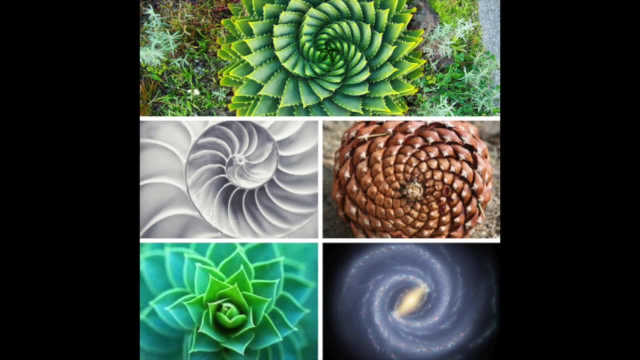 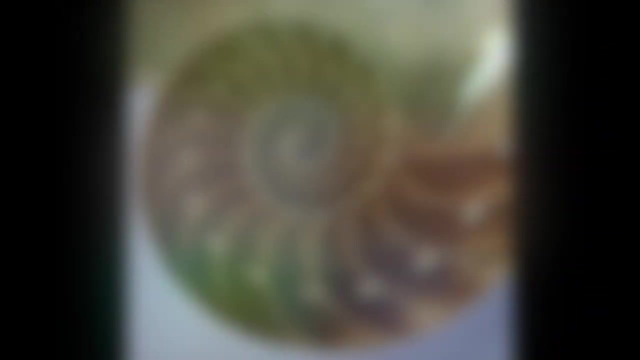 you ready to get started? Let's take a look at fractals. Fractals are found everywhere in nature and math. Fractals are patterns that repeat forever. They are created by repeating a simple process over and over again. You see the 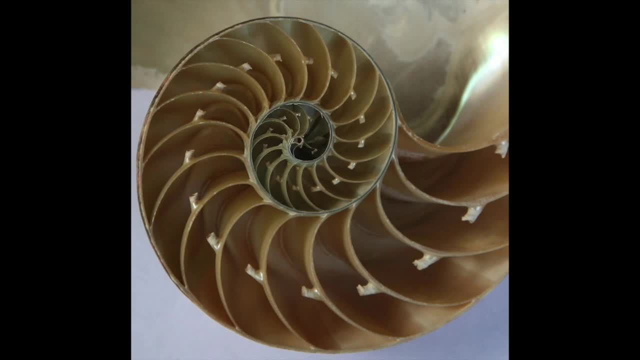 inside of the shell, How there's a shape all the way in the middle, in the center of it, and it repeats over and over again. It starts out small in the center and spirals out, But that same shape. you see those lines. It repeats over and over. 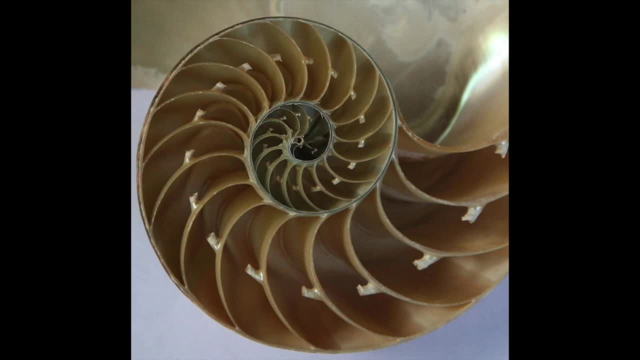 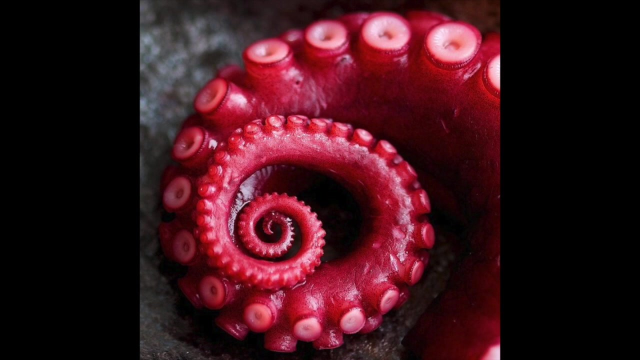 again. and as it repeats, it gets larger and larger, but it's still the same shape over and over again. That's what makes it a fractal. You see this octopus tentacle Again. just like the shell, it starts small in the center and spirals. 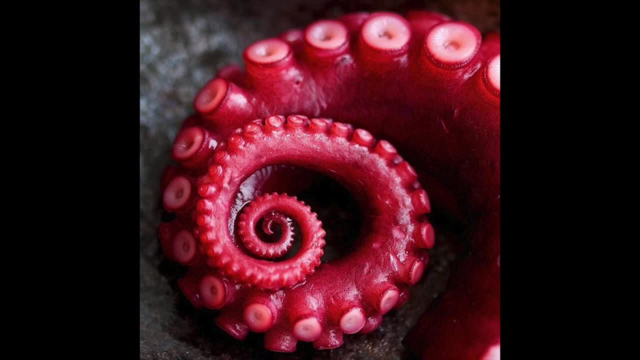 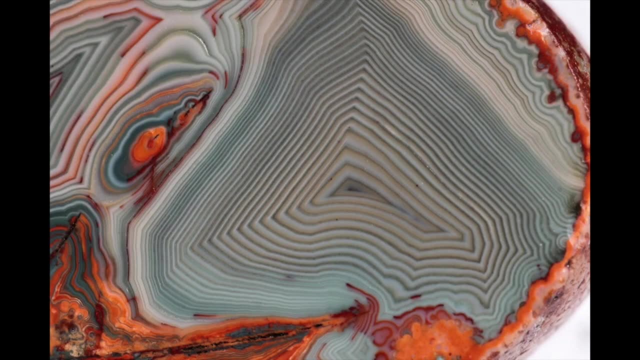 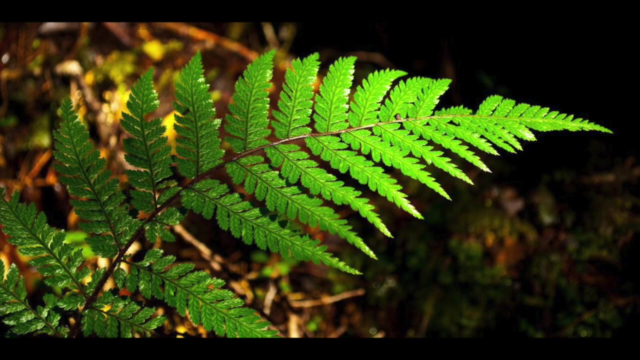 out. It's still with the same pattern, repeated over and over again. And same with this rock formation. You see, in the center It has a similar shape that repeats. You see how the leaves on this fern repeat over and over again. Fractals are found in tree. 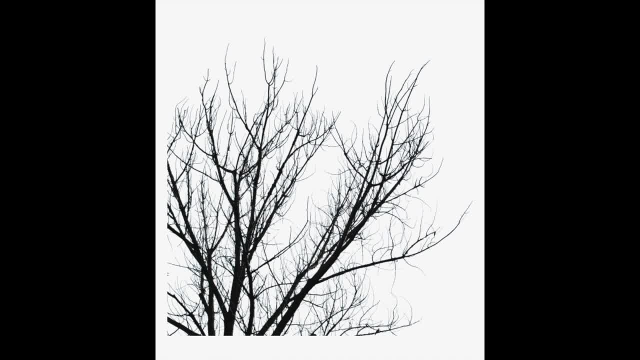 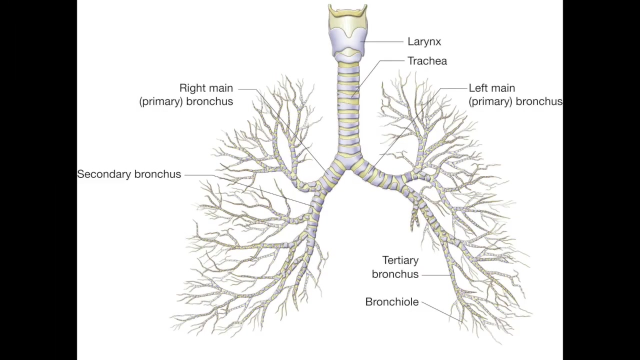 branches. If you were to take one part of a branch from a tree, you would see that it's very similar to the larger branches. Because tree branches are fractal in nature, Their growth repeats over and over again in similar ways. Just like tree branches, we have a similar structure inside our bodies. 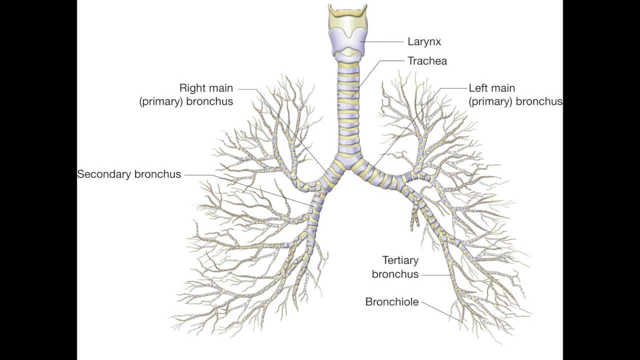 Here's an example of one of those. This is an example of lungs. You see that there are these branch-like formations And those are branches that repeat over and over again, in similar ways to tree branches. You see how they start larger and then, as you move out towards the edges, smaller and 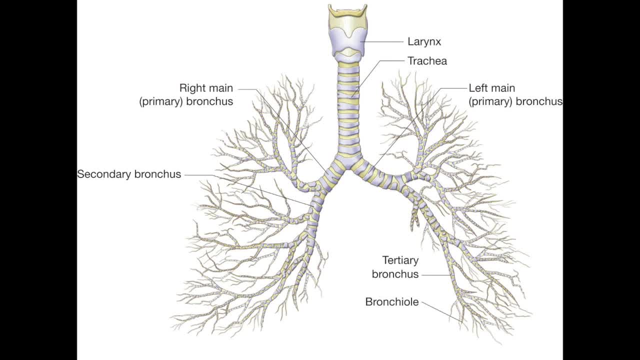 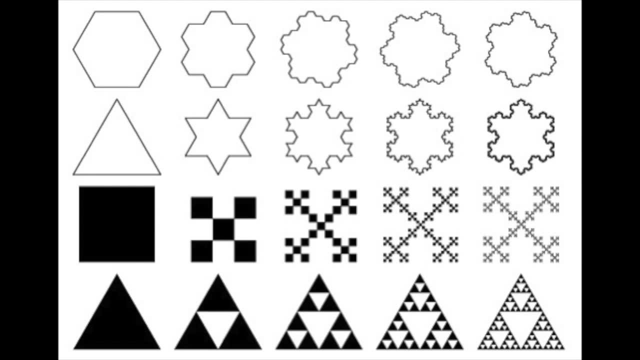 smaller. But you see the same kind of branch formation is repeated over and over again. In math, simple shapes are patterns. You see in the bottom row how a triangle, by repeating over and over again, makes a fractal. It starts off with a solid triangle on the left. At the very end. you get a series. 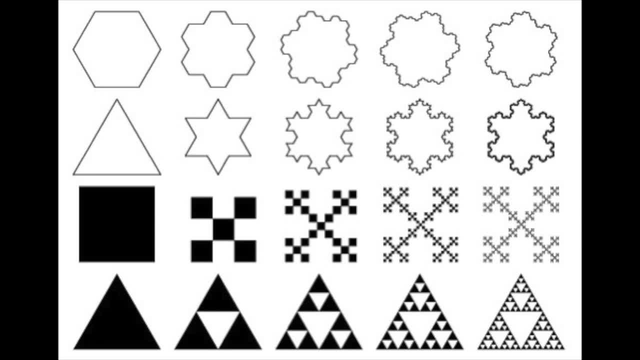 many, many different triangles all in that triangle, And that's an example of fractals, a repeating shape that creates a pattern. And you'll see in the row above it that there's an example of a square. It repeats over and over again to create fractals. 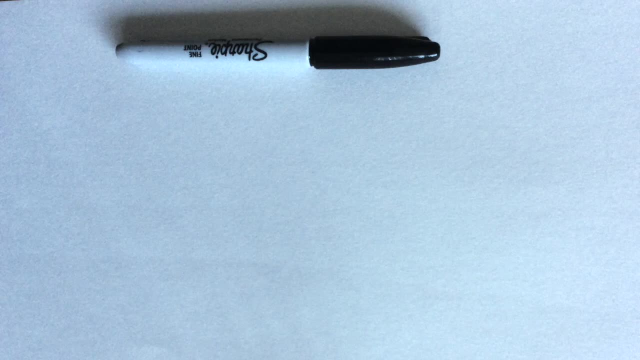 Now, the artwork we're about to do is inspired by fractals. Alright, so what you're going to need for this is a piece of paper and black marker. Now we will be doing six different types of drawings, so if you do want to have a total of six pieces of white paper, that's fine. 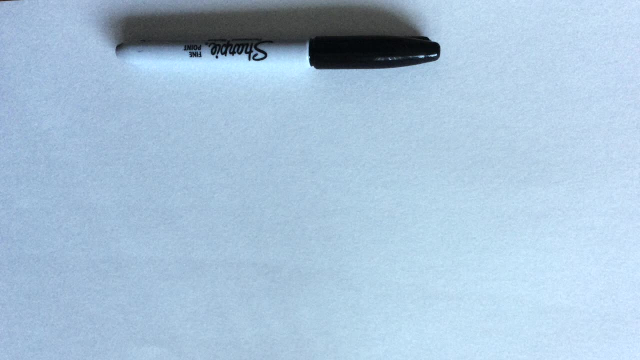 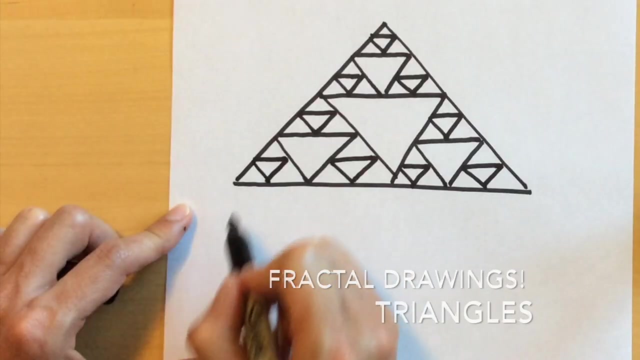 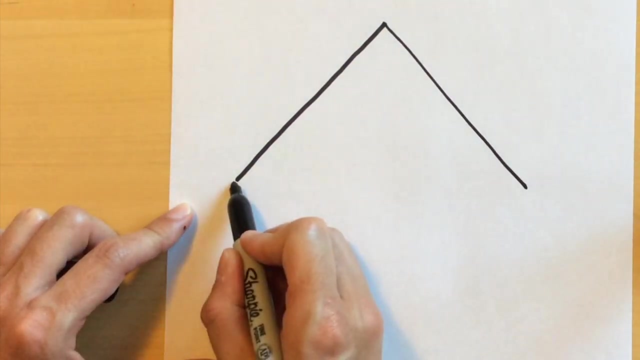 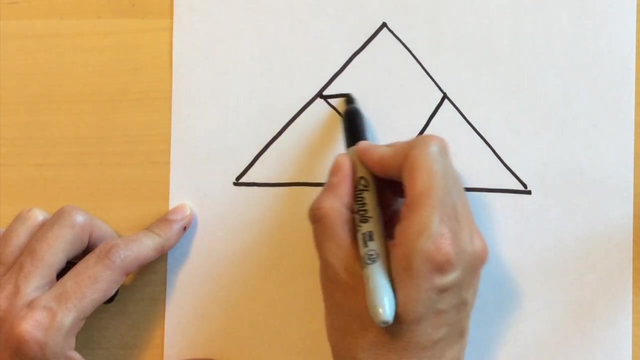 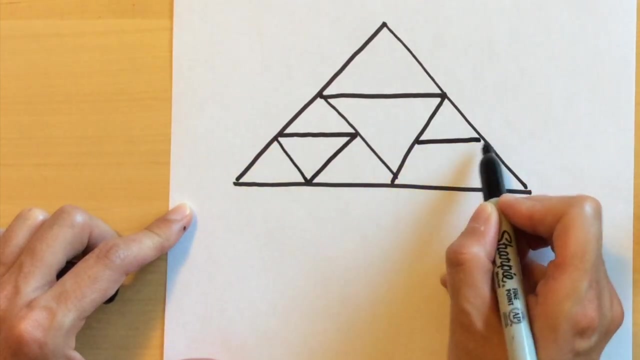 For each one of these exercises. If not, you can choose which one you want to follow, Or you can try creating them all on one piece of paper. That is your choice. Here we have the mixed paper and the together paper. This paper is going to go into the box. 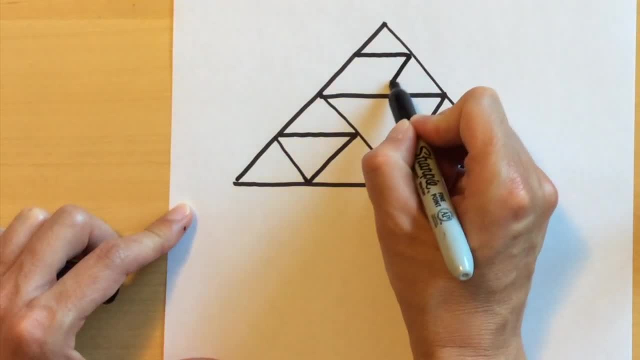 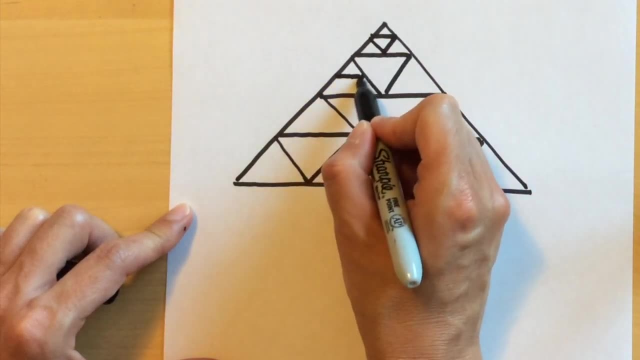 By doing this, we're going to make four different types of shapes. One of each type of paper is going to be made of white paper. Look, you'll notice that you'll get to pick up two different types of white paper to start working on. 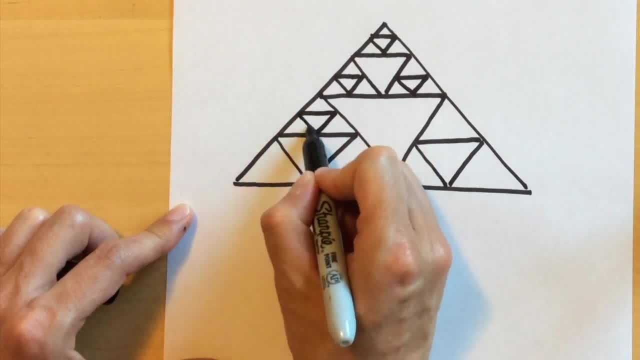 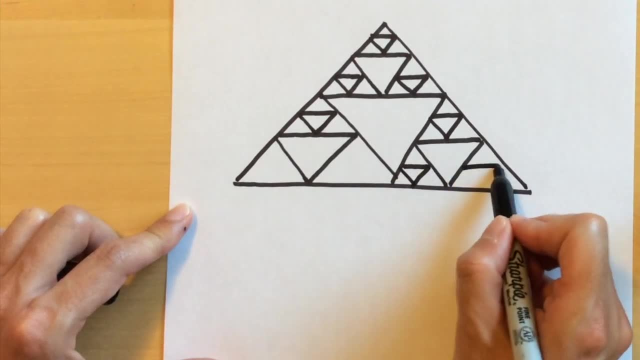 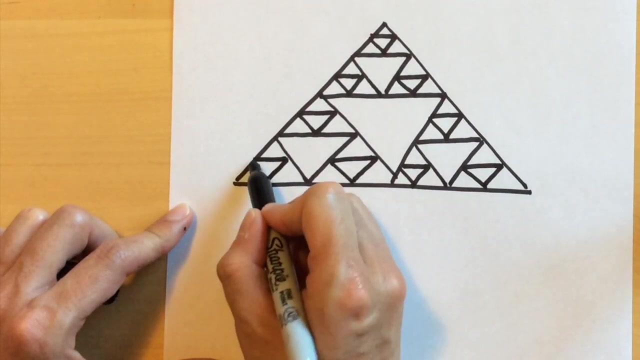 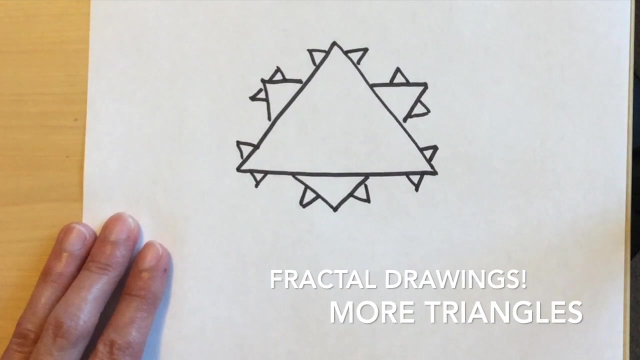 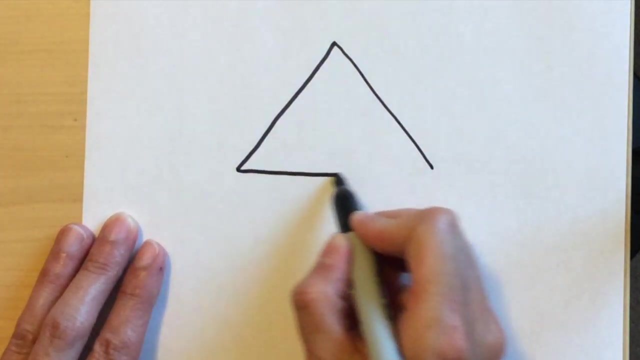 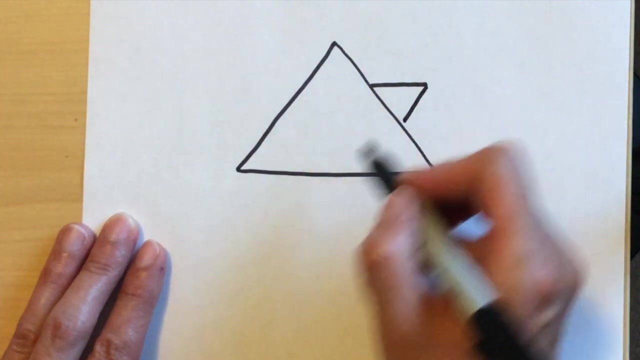 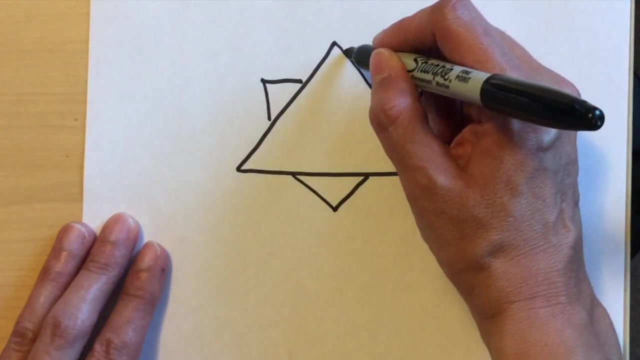 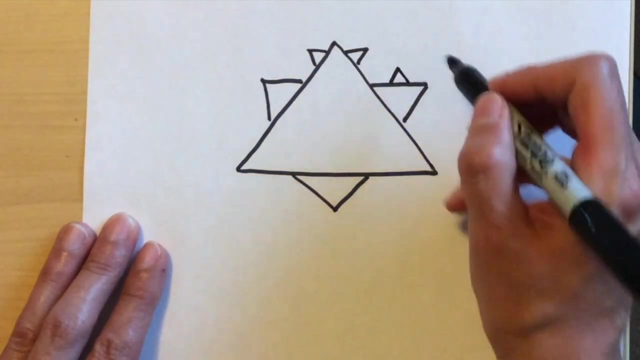 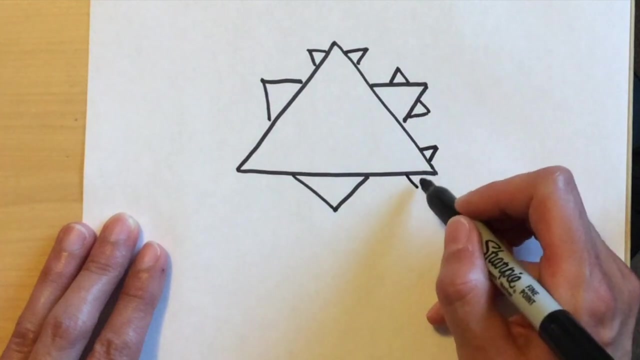 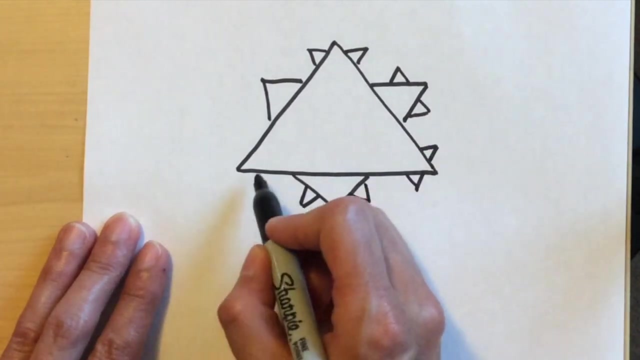 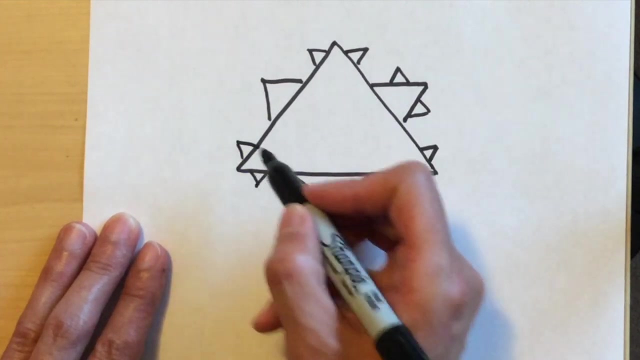 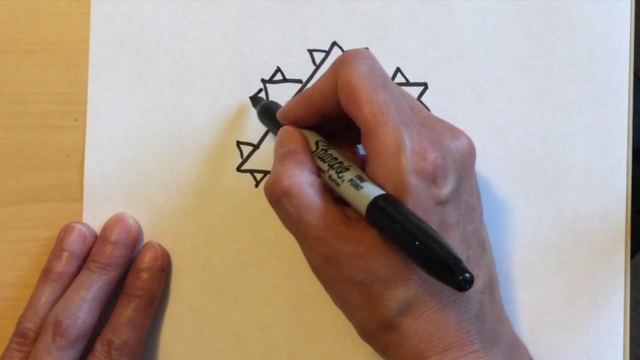 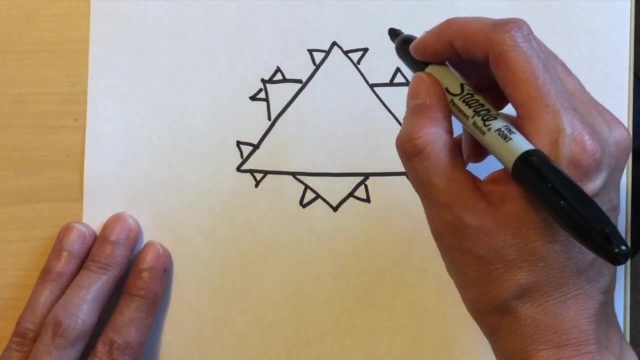 Now we are going to use two pieces of paper. as we start on the next piece of paper, Look, you'll notice that you'll get to pick up two different types of white paper to start working on. Thank you, Thank you, Thank you.